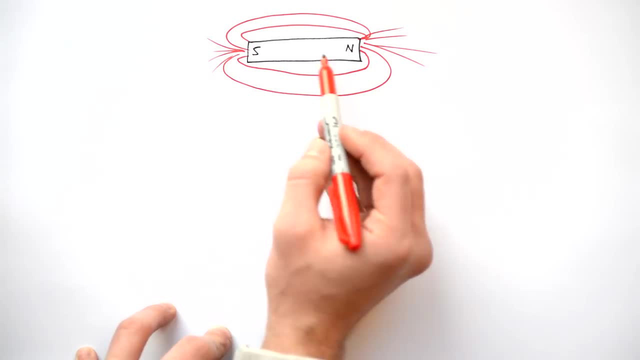 So they are always one complete loop. So that must mean that inside of this magnet all of these field lines actually carry on and they create a whole loop. That also must mean that these field lines that come out here must ultimately come around to the other side. 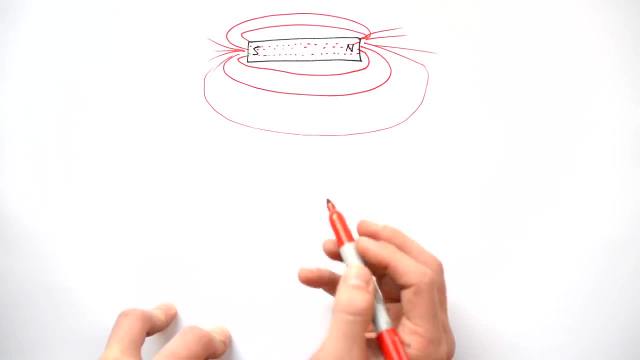 as well. The direction of these field lines always go from north to south, So we can draw arrows on them like so. You probably also know that when you have two magnets that are next to each other, when you align them in the same direction. so the north pole of this- 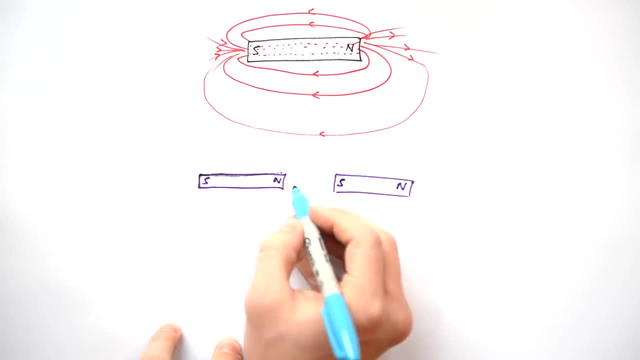 magnet is facing the south pole of this one, they actually attract each other. If we were to draw lines, we know that field lines go from north to south, So they would actually just go straight from this pole of this magnet to the south pole of this one. Ultimately, what you'll find is that 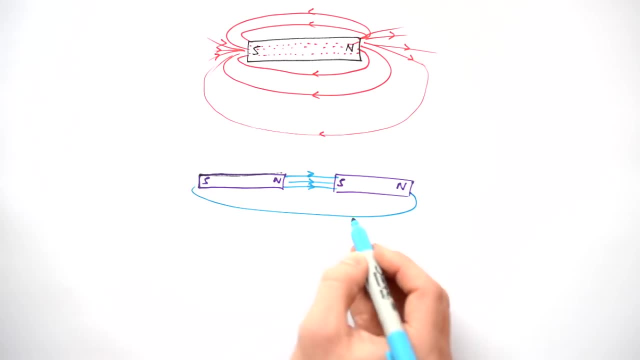 you've made a big magnet using these two magnets. Again, these field lines are unbroken, They're just invisible, as it were, inside of these magnets. again, Lastly, we have two magnets whose poles are facing each other, so north and north. 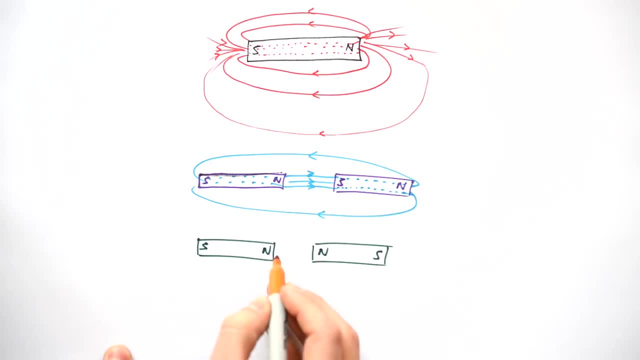 Then we know that the field lines can't go from north to north pole, but also they're not going to be flying out like the top one up here, because this magnet's getting in the way. What happens is that if you bring two north poles together, the field lines will almost touch the middle. 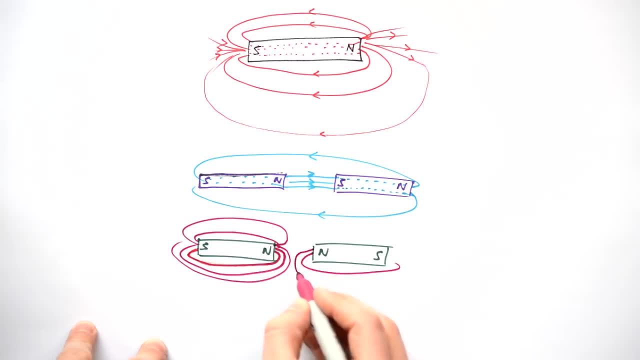 but they're not going to be flying out. So you can see that the field lines are getting more compact because they're being repelled by the field lines from the other magnet. The closer you get these two magnets together, the more dense these field lines become And you 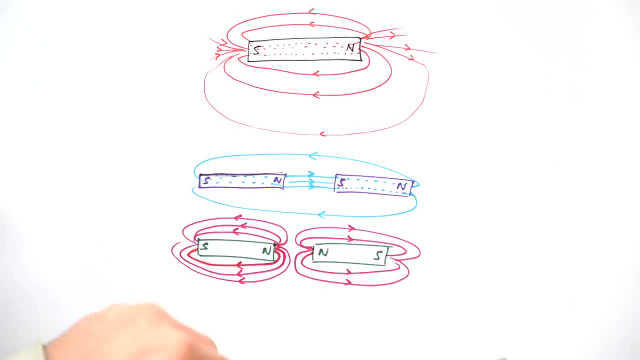 probably know that the closer you get them, the bigger the force that's trying to push them apart. That's actually a really important point. is that the more dense the field lines, the more dense the flux density. We'll get onto what that means in a minute. I'll get onto what that means in a minute. 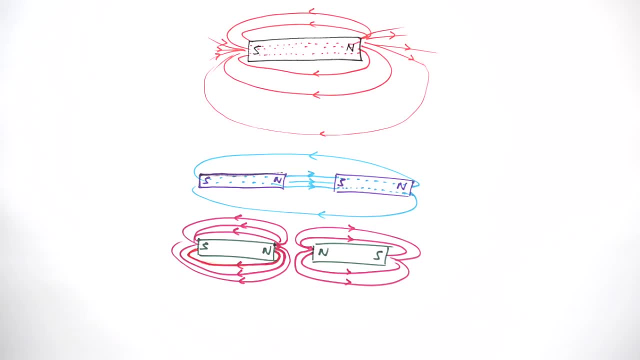 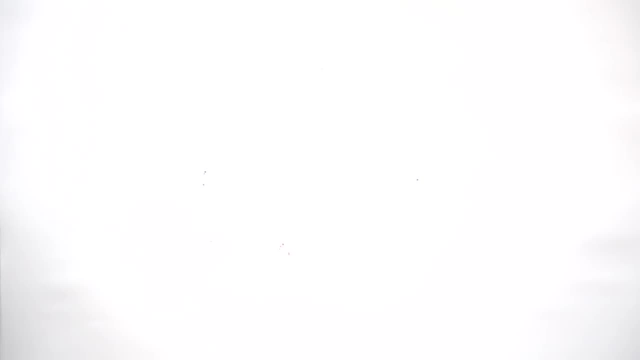 That means the bigger the force the certain objects are going to feel at those points. Let's take a step back, though. What do we mean by north and south pole When magnetism was discovered, that such materials actually lined themselves up so that one end of an object pointed towards the north pole of the earth? 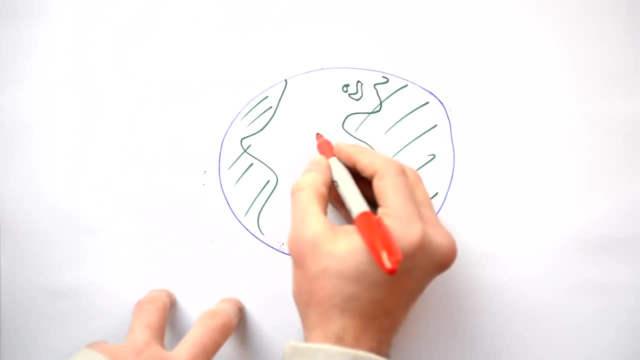 and the other one pointed towards the south pole of the earth. So what did they call these two poles then? They called them the north pole and the south pole, The north facing pole and the south facing pole. That's where north and south comes from. 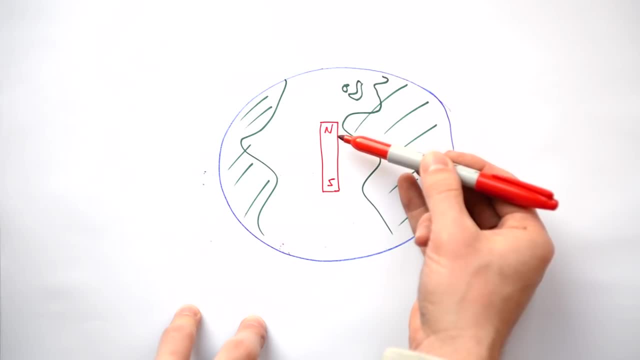 So we write n or say north pole for short, but in reality that means north facing. This means south facing Again. we know that these field lines go from the north pole of the magnet, that's the north facing pole of the magnet, to the south facing pole of the magnet. 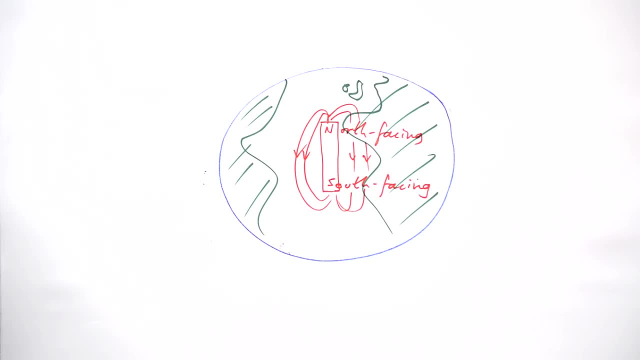 Here's where it gets a little bit weird, though, As the earth acts as one giant magnet as well. that actually poses a problem, because we know that two north poles will repel each other. So this here is geographical north, this is geographical south. 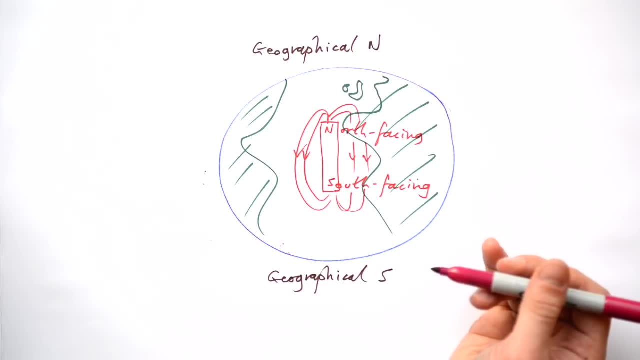 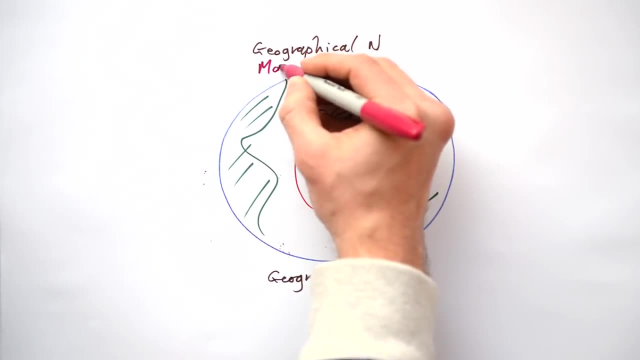 But if the earth does act like one giant magnet, then that must mean that in fact, the geographical north and north pole of the earth is actually its magnetic south. Unfortunately, there really is no way around this. It's just something that has to be true, but it's really important. 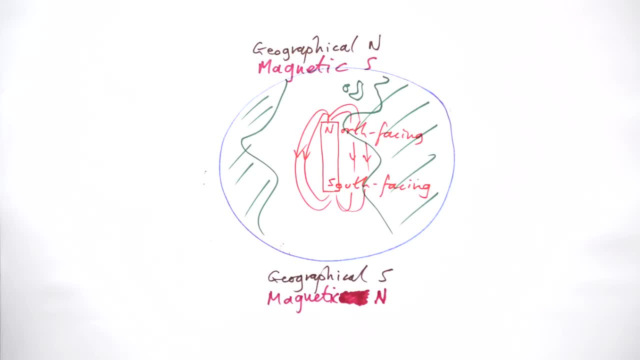 Therefore, which way do the field lines go for the earth? They actually go from the Antarctic to the Arctic. That has to be true if we want our magnets to line up the right way in order to call them north facing and south facing. But from now on we're going to drop the facing part and just call them north and south poles. 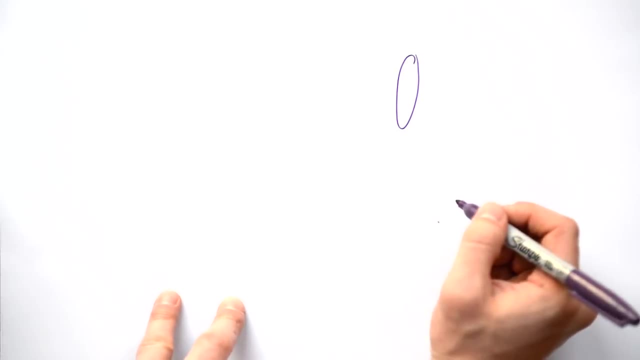 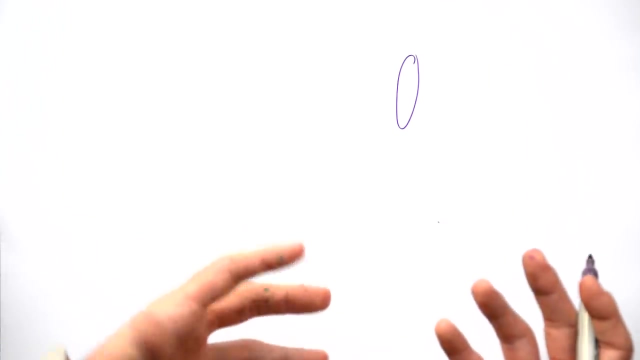 If I have just a circle, a certain area, and I want to know how much magnetism I have going through it, in other words, how many field lines, as it were, then I can draw my magnetic field lines going through like this: 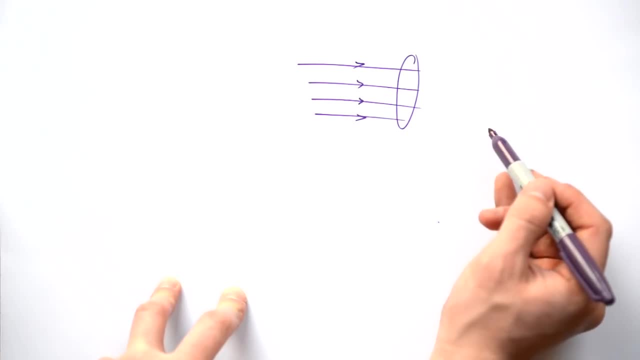 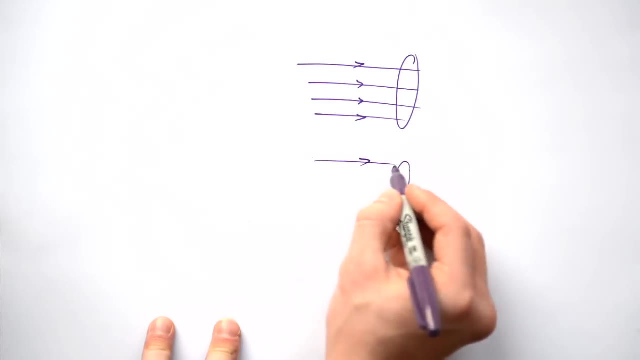 I know there has to be a north pole over here somewhere and a south pole over here somewhere, because field lines go from north to south, but I don't have to draw those. What about if I draw the same thing and then I draw these field lines going in? 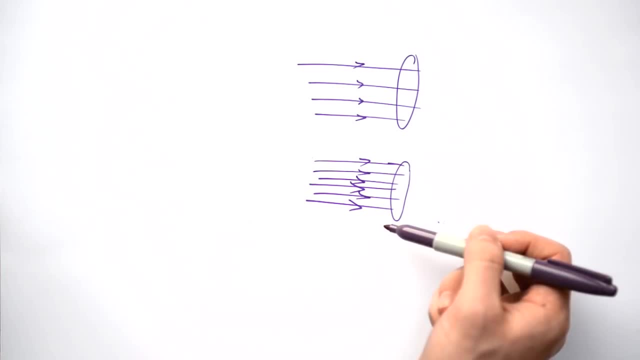 We can see that there are more field lines closely packed together, so that must mean that we have more magnetism, as it were, And we call this amount of magnetism flux. It has the symbol phi, which is a Greek letter, and the unit is Wb, which is short for Viber. How tightly packed together is my magnetism here compared to here? Well, let's say that these field lines here are twice as compact as these field lines here. I can say that the flux density here is greater than the flux density here. How tightly packed together are these field lines, this flux? 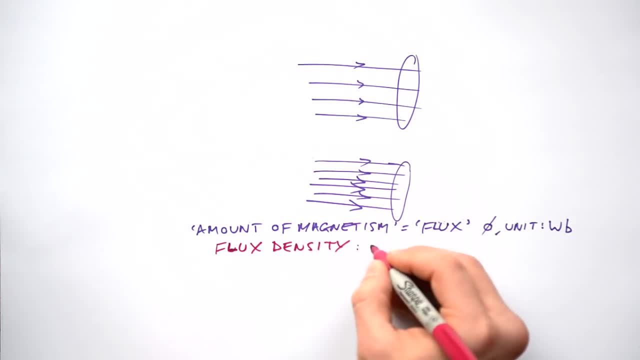 We call this flux density and it's given the symbol B and it has the unit T for Tesla, named after Nikolai himself. How do flux and flux density link together? Well, when we talk about density of materials, we take the amount of mass and we divide it by the volume that it takes up. 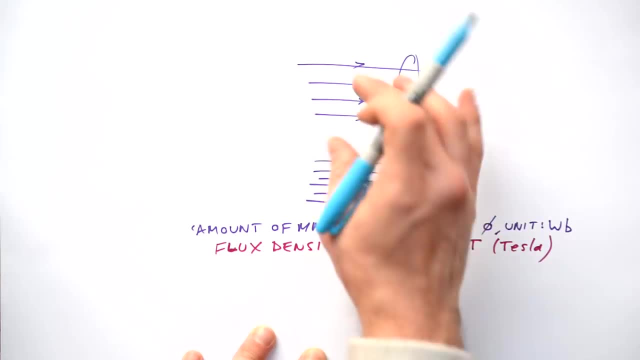 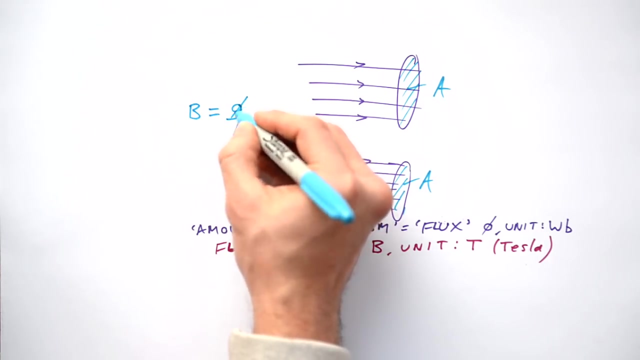 In this case we're not dealing with a volume, though. we're dealing with an area. So how much magnetism, how much flux is going through this area? here I'm going to call that A Flux. density is equal to the flux divided by the area. 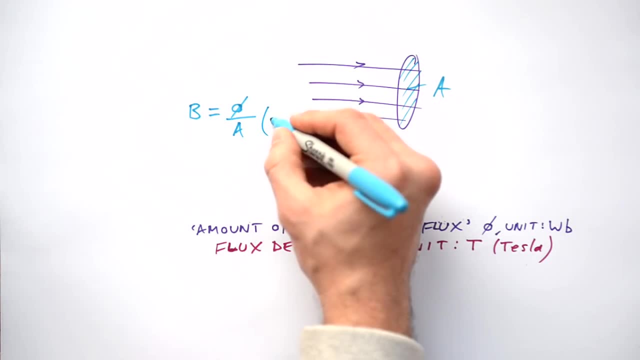 So you might be able to see that the alternative unit for this is going to be Vibers per meter squared. That means, therefore, flux is equal to B? A, And this is an equation that we're going to see in the circuit time and time again. 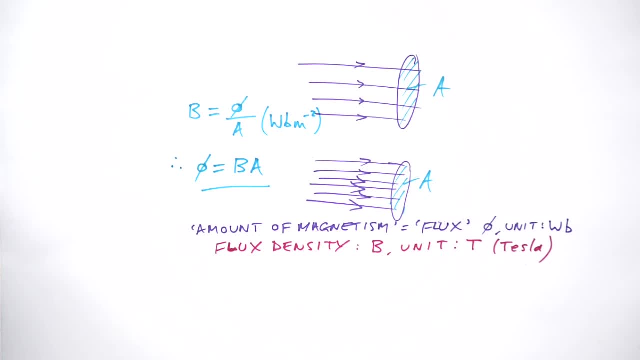 Electricity and magnetism are very closely linked. They affect each other. If you have a piece of wire and have a current flowing through it- I'm going to call that I- then you might know that that will create its own magnetic field around the wire. 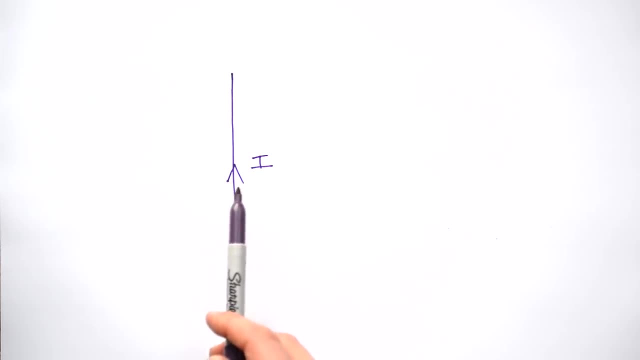 Whenever we have a wire and we draw an arrow showing current, this is actually what we call conventional current. This is the opposite way to which the electrons are flowing in the circuit. That's something that's very important later on when it comes to free moving charges. 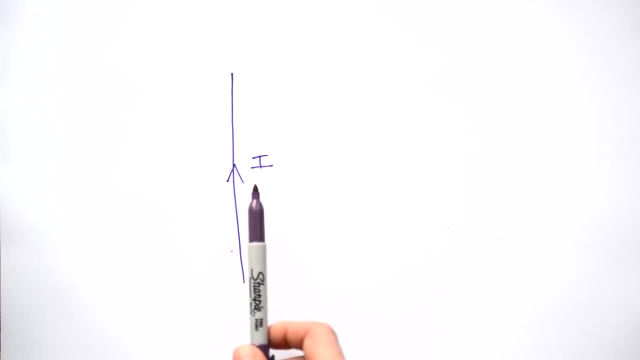 You can think of conventional current as the way that positive charge moves in a circuit. This actually creates a circular magnetic field which form continuous loops around the wire. But which way are the field lines going? Are they going this way here? so it's anti-clockwise. 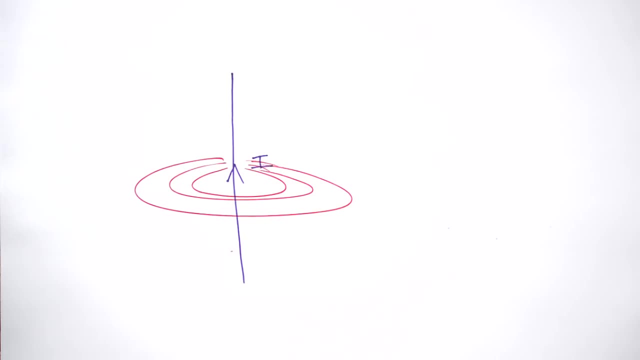 or this way clockwise. Well, Maxwell came up with a rule called his right hand rule or the corkscrew rule. So you've got your hand like this and you curl up your fingers like that. Your thumb is the direction of the current. 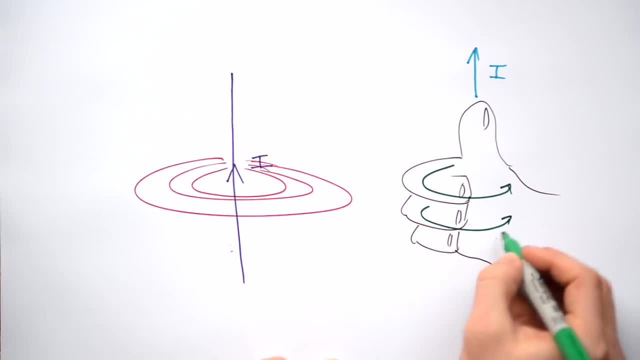 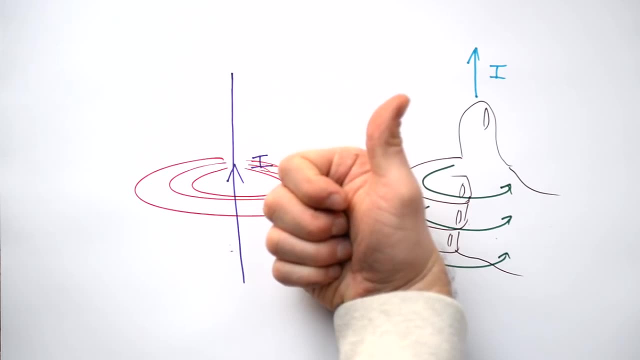 and the way your fingers curl round is the direction of the field. We can see in this case that the current is going upwards. Get your thumb, curl your fingers round like you're putting a thumbs up, and we can see that the field line should be going that way, around the wire. 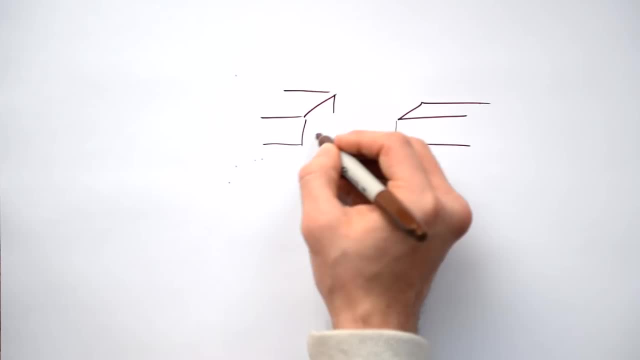 If we have a magnet, two magnets, with a gap in between, like so Let's say, this is the north, This is the north pole of this magnet, This is the south pole of that magnet. We don't have to draw the other poles because we're not concerned with those. 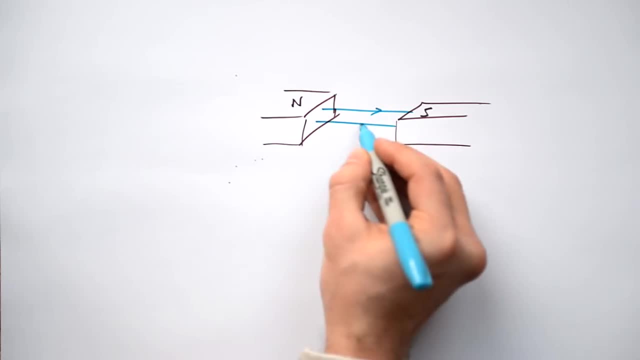 Which way would the field lines go? Well, they should go north to south. If you actually take your wire with the current flowing through it, like so, and you put it in this magnetic field, because this wire with the current produces its own magnetic field. 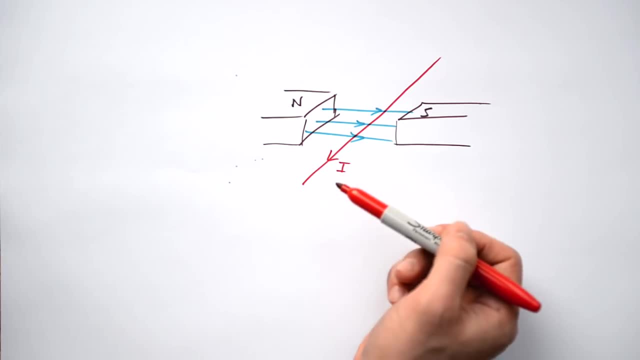 we actually have two magnetic fields that now interact with each other. What we'll find is that the wire will move because there will be a force which acts on the wire. If the wire was held still, then the magnets would move in the opposite direction. 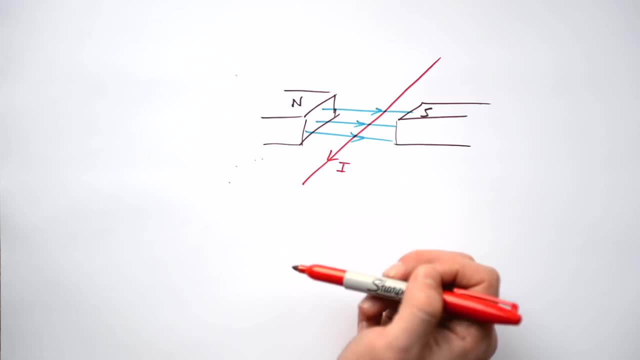 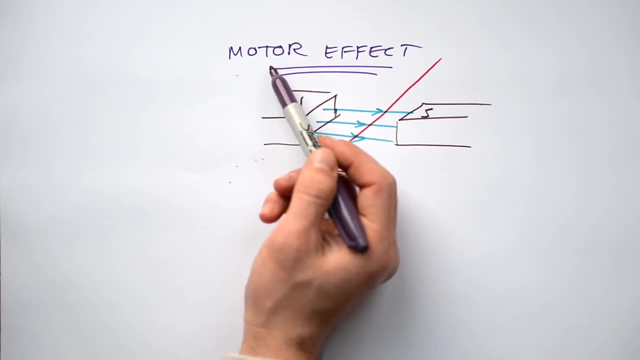 But for now let's just think about the magnet staying in place and the wire being free to move. This effect is called the motor effect. Whenever you see motor, that means that something is going to be moved, and that's what's happening here. 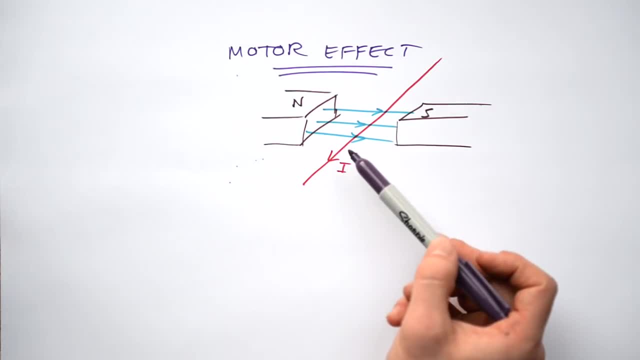 We have a current in a wire that's in a magnetic field, and that wire is going to move. But which way is it going to move? Well, we need another rule using our hands, but this time it's Fleming's left hand rule. 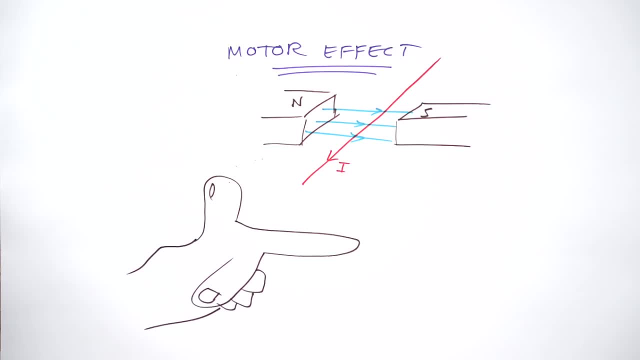 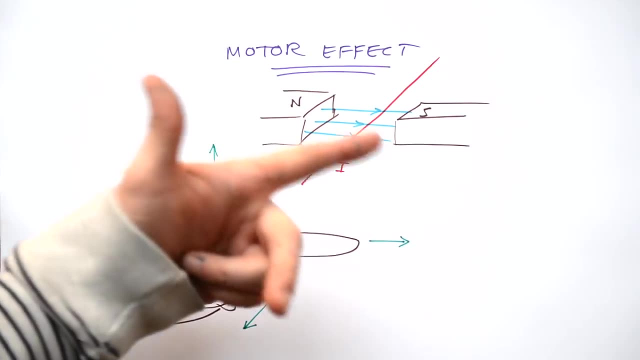 If you can't tell, that is actually a hand that I've just drawn and we're only concerned with the thumb, the first finger and the second finger. Now, this is in 3D, so we're talking about the thumb going upwards here. 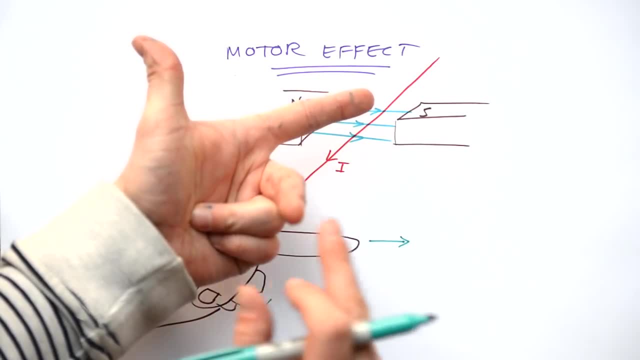 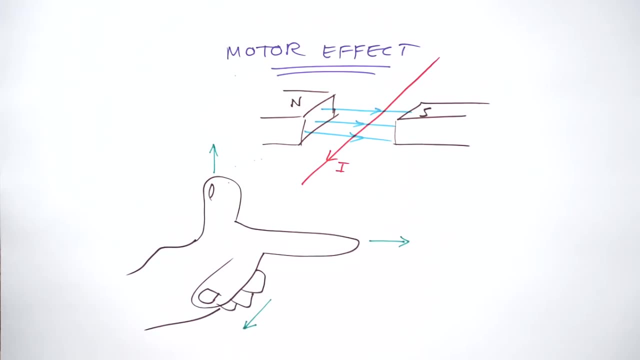 first finger going to the right and the second finger here actually coming out towards me, Coming out towards the camera. So, if I can put it like that, you can see Now the easy way to remember which finger represents what in this situation. the first finger begins with an F. 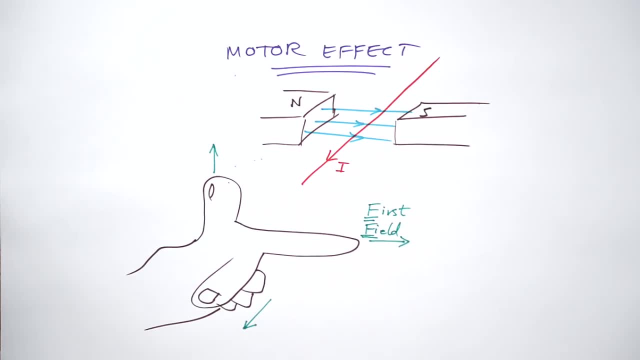 and that actually tells you the direction of the magnetic field. The second finger has a C, and that indicates that that's the current. It's not the most convenient way of remembering, but it will help. And then, finally, we have the thumb. 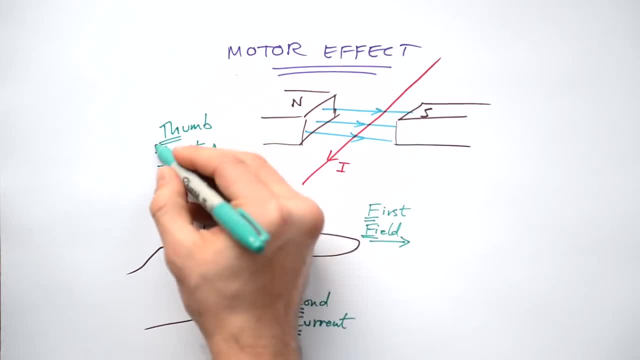 which is the thrust, Obviously. that's what the force is. That's the direction that the force is going to be exerted on this piece of wire. Which way is this wire going to move? I can see the current is going that direction. 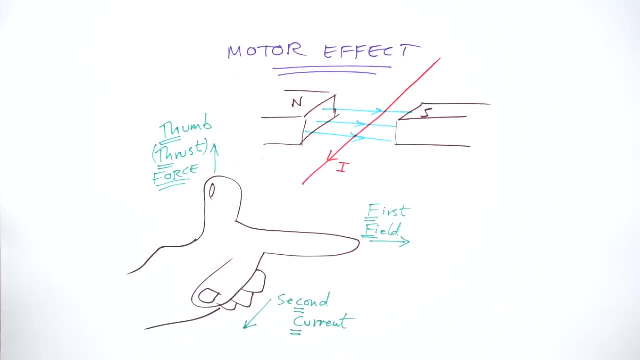 field is going from north to south in that direction and my thumb is pointing upwards. So that means that the force is going to be upwards, The wire is going to move upwards due to the motor effect. But there is also, Fleming says- 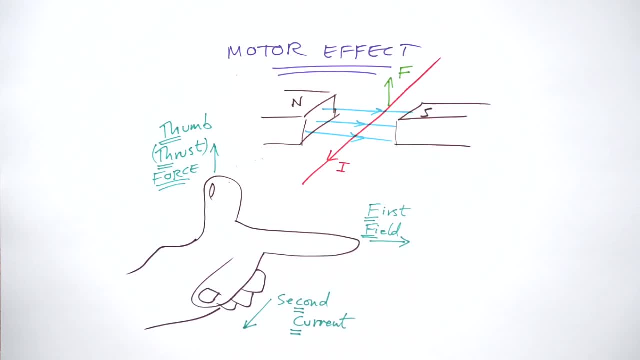 Wendy says right hand rule as well, But the left hand rule is used for the motor effect. How can we remember this? Well, the way I remember it, motor cars drive on the left, At least they do here in Great Britain. I'm sorry if you're in a place where cars drive on the right hand side, but in Britain that's how. 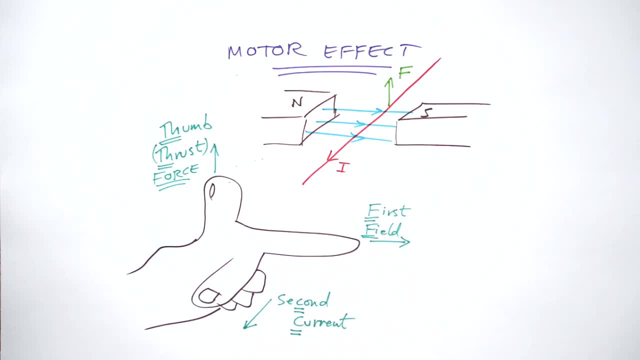 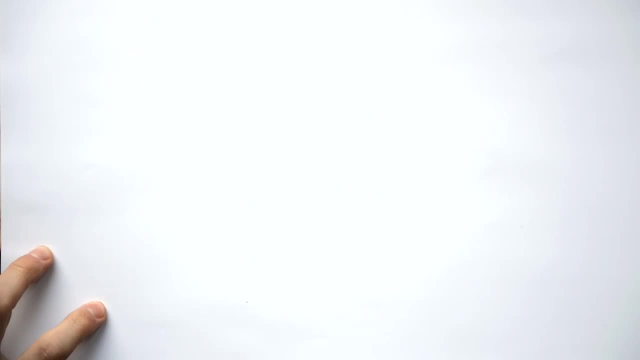 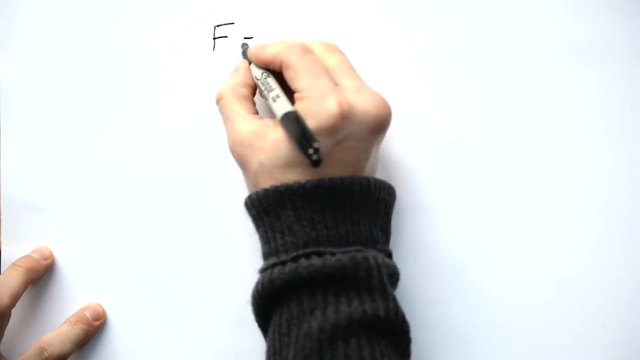 we can remember it, Motor cars drive on the left. so when we are dealing with the motor effect, that's, force being supplied to a wire carrying a current, we use our left hand rule. So how can we calculate the magnitude of the force, How many newtons? It's as simple as f equals b, i, l or f. 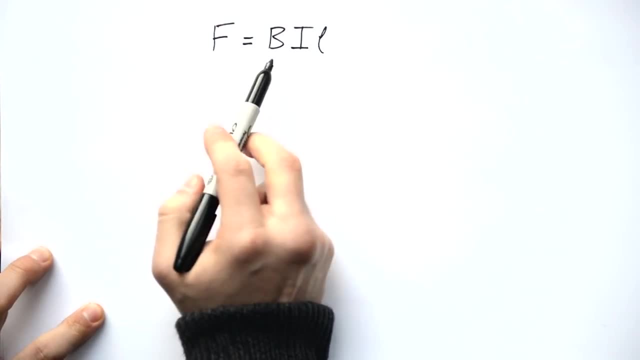 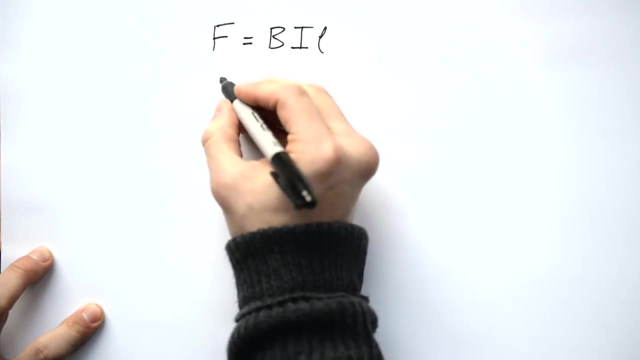 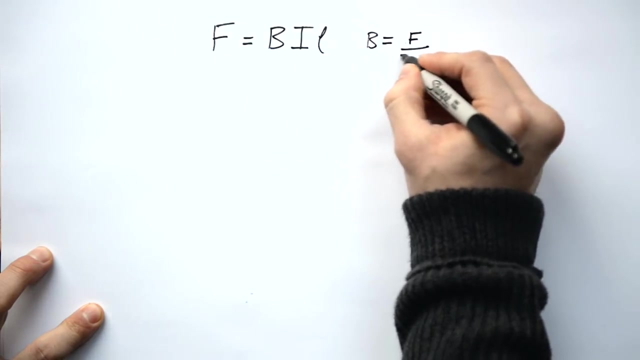 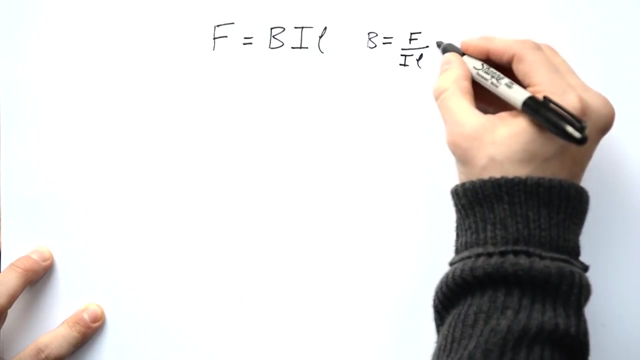 so the force on a current carrying wire is the magnetic flux density times the current times, the length of the piece of wire. Incidentally, as an aside, if we rearrange this for b, we find that flux density is b force over current times length. So an alternative unit for flux density is newtons per amps per. 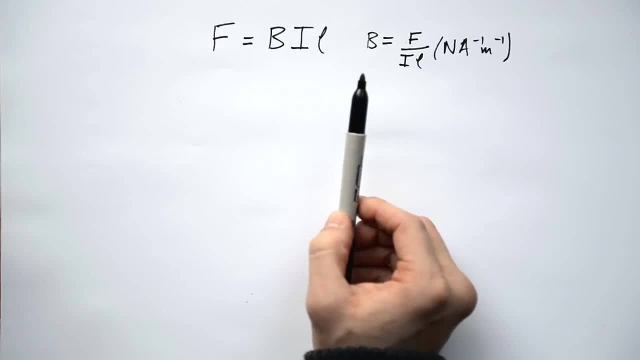 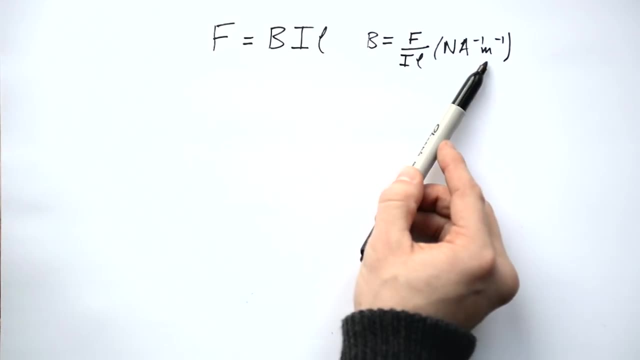 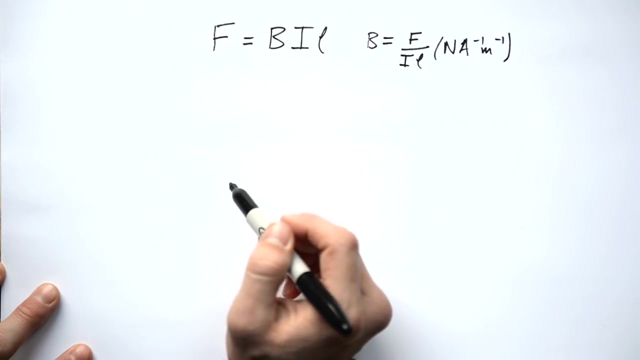 meter. This gives us another insight into what flux density is and how it can be calculated. Flux density is the amount of force exerted on a piece of wire that's one meter long carrying one amp of current. This is only true if the current and the flux density are at right angles to each. 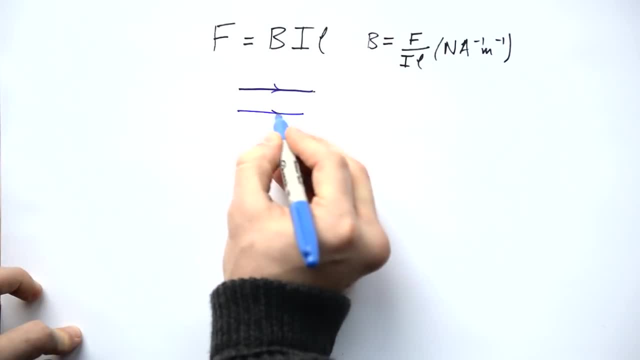 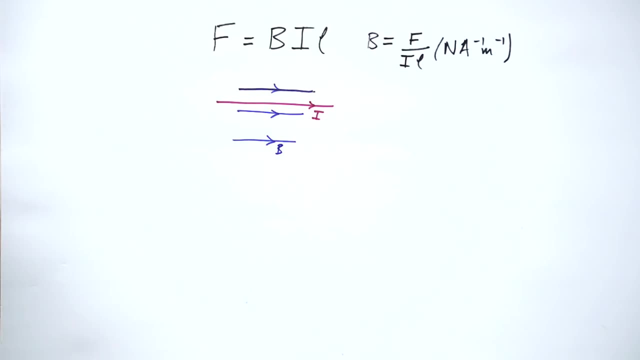 other. like with Fleming's left hand rule, If the field and the wire are both in the same direction, then we have no force. So they have to be perpendicular to each other and you might realize that if the wire was at an angle then we'd have some component of f bill and that would be times cos theta. But we'll leave that one for now. 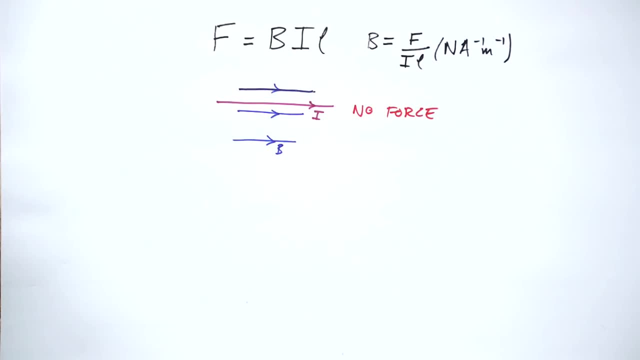 Because we're dealing with three dimensions. we actually have to find a way of representing three dimensions on a 2D plane, a piece of paper. If you're drawing in 3D, then we need to think darts. If you have a dart like so, what do you see if a dart is coming towards you? 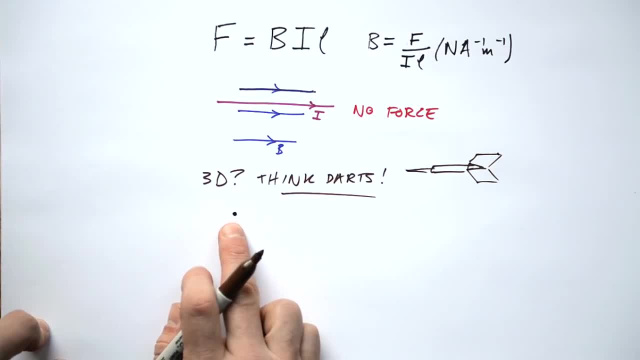 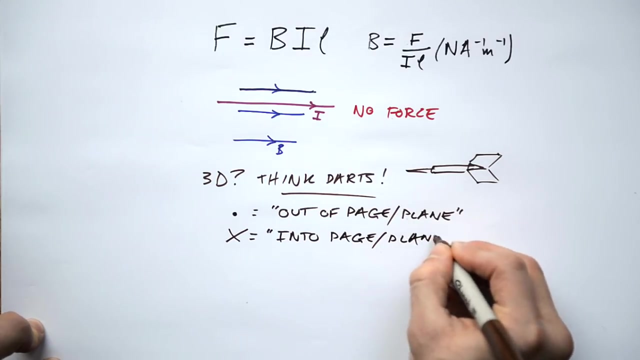 You see just the tip. And so if we draw a dot, that means that the dart is coming out of the page or out of the plane. If a dart is going away from you, what do you see? Well, you see the cross of the flight. So we say that's into page or plane. 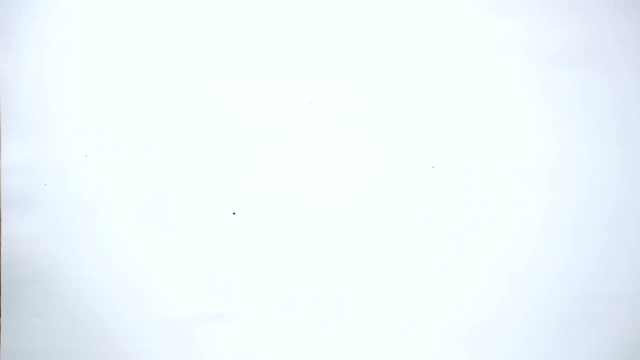 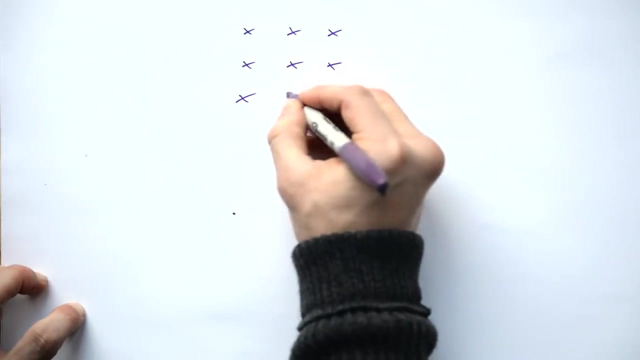 More often than not, it's the magnetic field that will be drawn using this dot and cross method. So let's say that we have a field going into the page. We draw a few crosses like that So we can say b, that's the magnetic field. 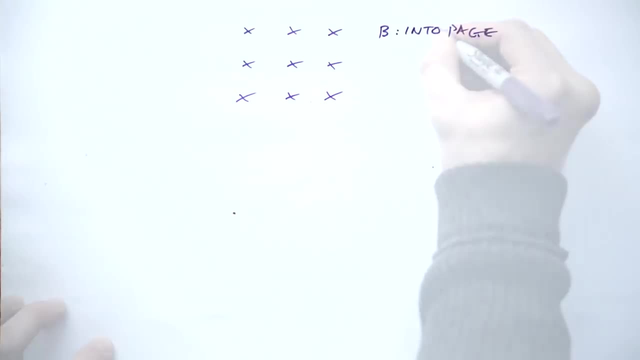 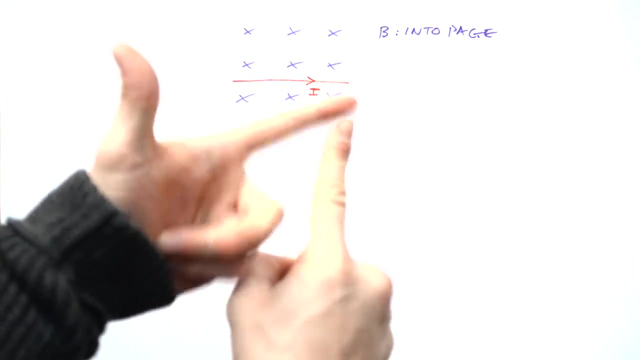 The flux density into page. Now, if you introduce a piece of wire with a current flowing that way, Again we're talking conventional current, That's the flow of positive charges, But in a wire we just call it current. Can you predict using Fleming's left hand rule, that's thumb thrust, that's force, first finger field, second finger current. 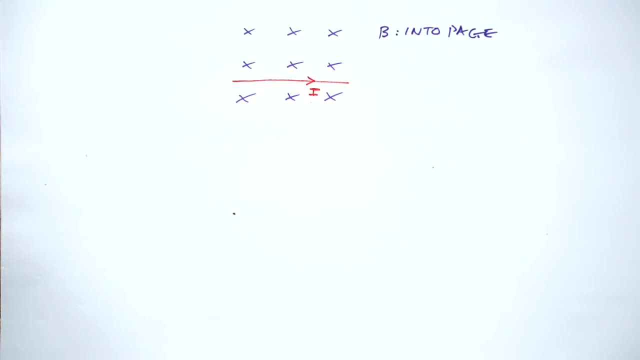 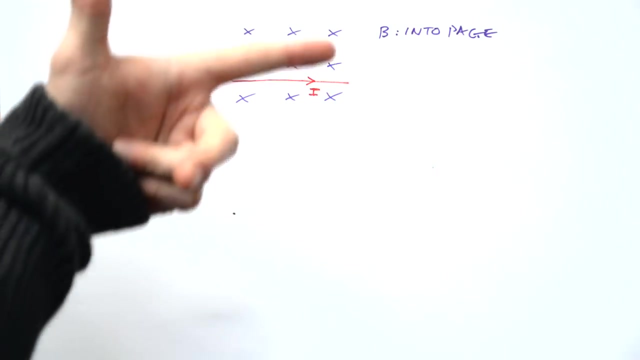 Can you predict which direction the force is going to be And therefore which way the wire is going to move in this situation? Give it a go yourself now. Pause the video if you need to. So if we orient our left hand, then we have the field going into the page. 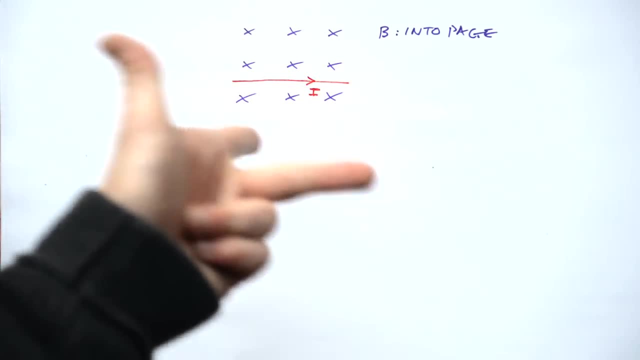 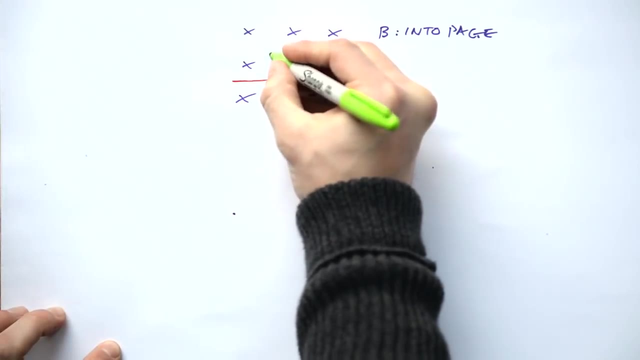 So let's stick our finger. that way That's going into the page. Our current is going to the right, so that means our thumb is left going upwards, So that means that the force is going to be acting Upwards, And that's how you deal with the motor effect. 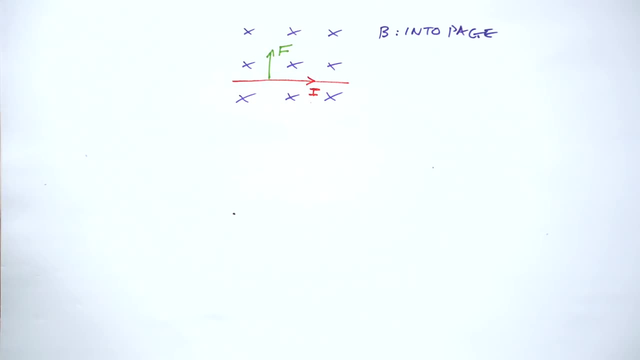 You can predict the direction and the magnitude of the force on a current carrying piece of wire in a magnetic field. So if we can find out the magnetic flux density of a magnetic field at a certain point by just measuring the force, The question is, how do we actually measure the force? 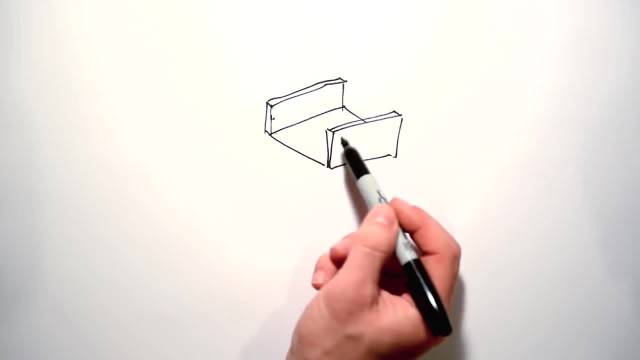 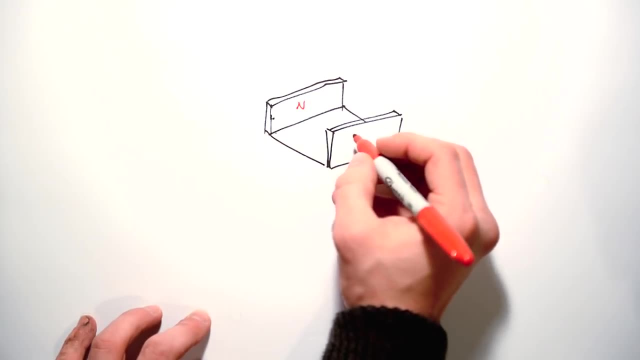 Well, there's a very easy way of doing it. What we do is get two magnets and attach them to a bracket, Just like this, And let's say that this pole here is north and this pole here is south. So we know that the magnetic field lines are going to go from left to right. 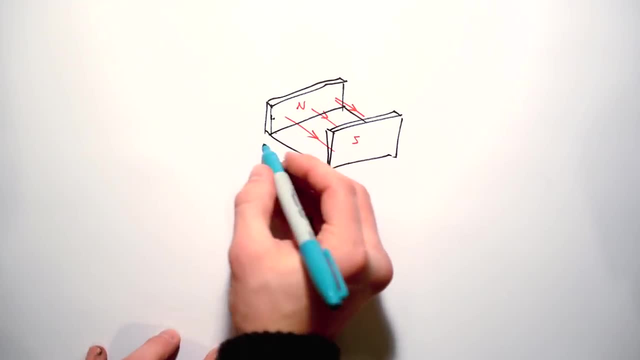 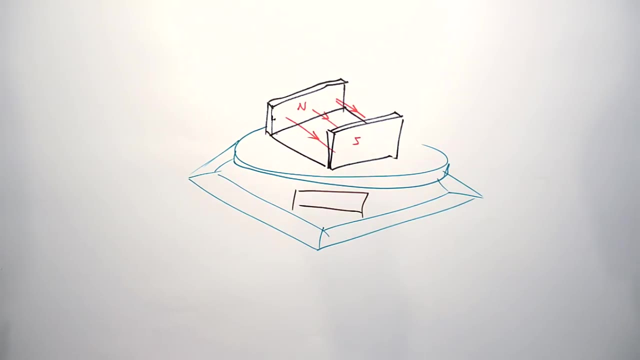 So if we put this on a top pan balance like so, And then we tear it first, So with nothing going on, we just have zero, zero kilograms on here after we've teared it, Then what we do is get A piece of wire. 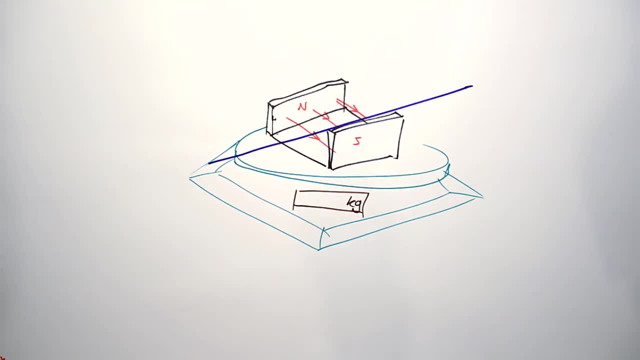 As part of a circuit And we pass a current through it And we put that directly in between the two poles. Now we know how long the length of wire between the two magnets is, Because that's just going to be the length of the magnets themselves. 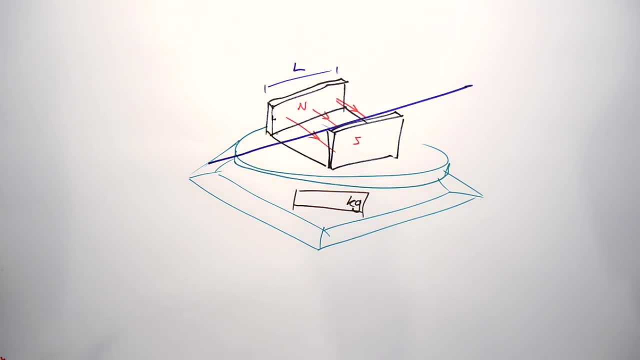 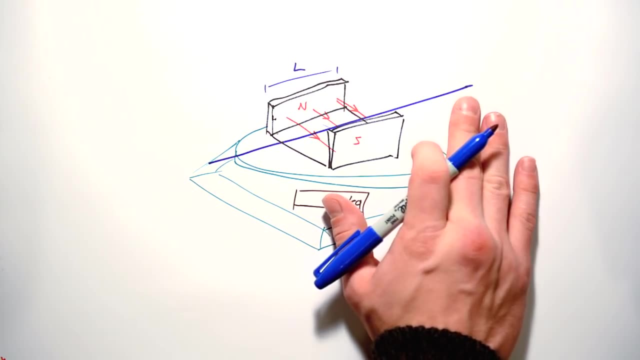 And we can measure the current as well. But before we put on the current, let's figure out which way we want this top pan balance. This wire is going to be clamped in position so it cannot move, If it can't move, But there is a force exerted on it. 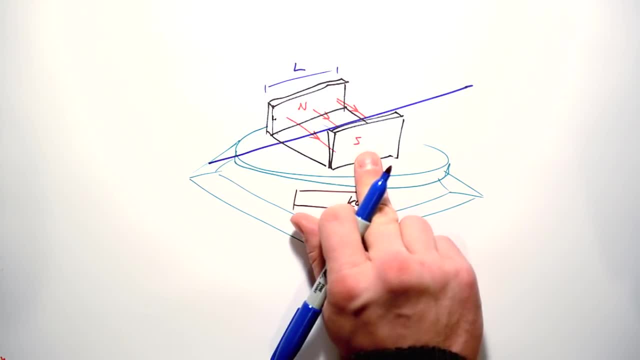 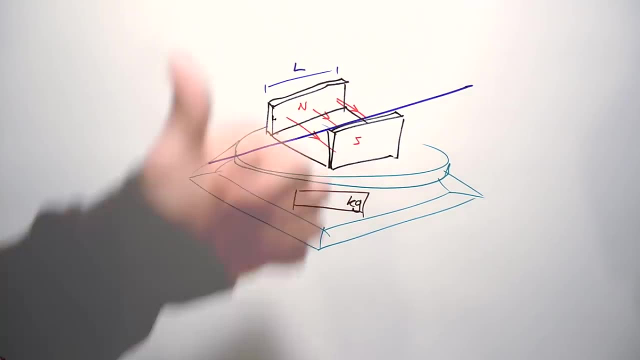 That means that there's going to be a force exerted on the magnets instead And they are going to be moved downwards. So let's have a think: We want the force to go upwards on the wire. See if you can predict which way we want the current to go in this wire. 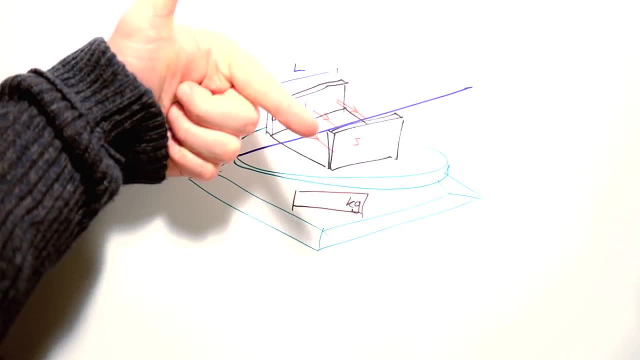 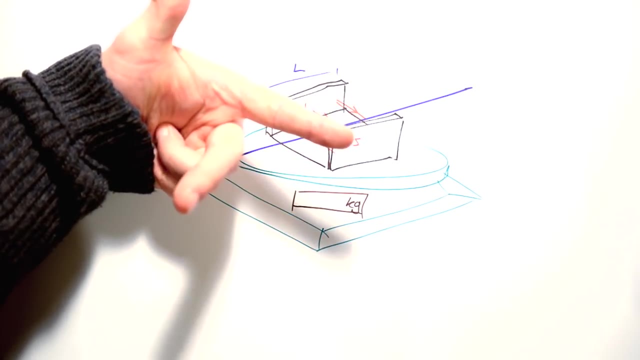 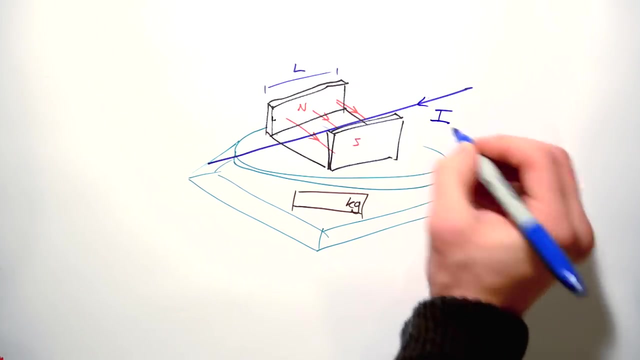 So we want the force to go up And we have the field going left to right like that. So we want the force going upwards. Field is going that way. Therefore, We want the current to be going this way through our wire. So that is the direction of our current. 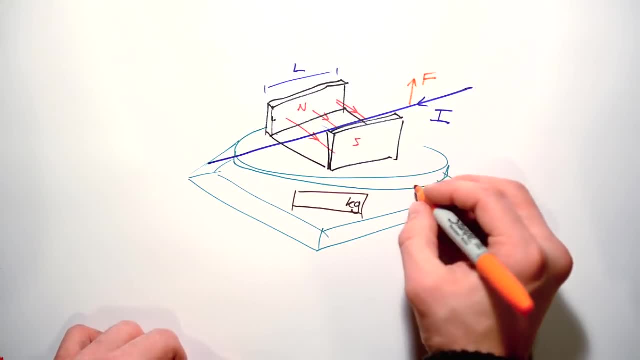 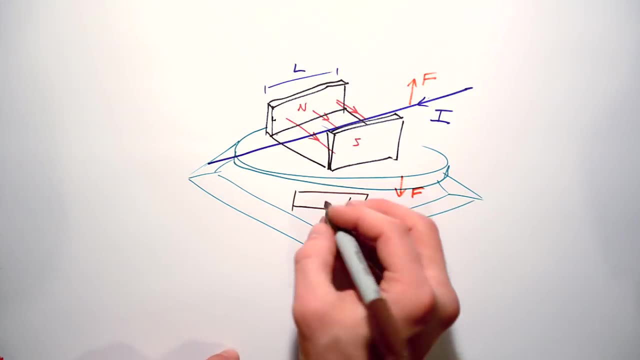 If we have a force pushing upwards on here, That means that we have a force pushing equally down on the top pan balance down here. So let's say that once it's turned on, Our balance actually measures a mass of that 0.05 kilograms or 50 grams. 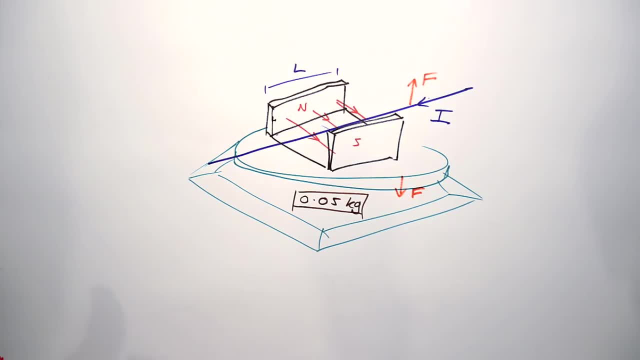 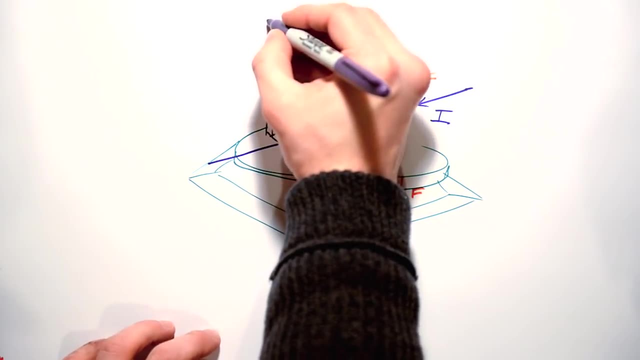 Now we know that that's a simulated mass. The only reason that the top pan balance says that Is because the magnets are pushing down more than they should do, Just from their weight. We can say that because we know that F equals BIL. 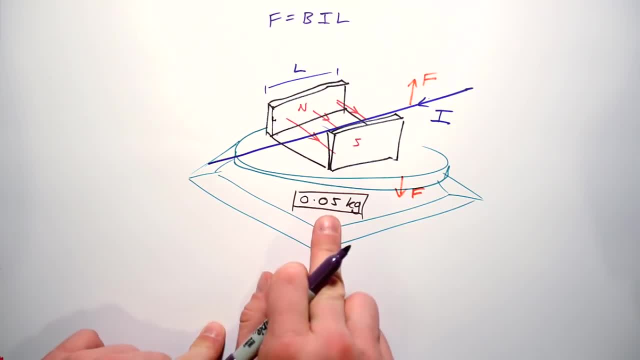 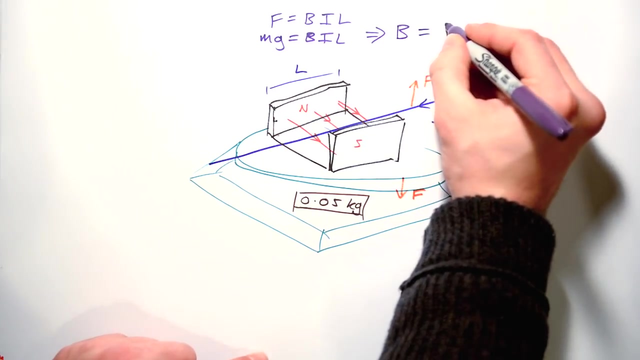 I'm going to use big L here. That means that if we measure a mass on here, We can say that MG equals BIL. Using this, we can just rearrange this To find that the magnetic flux density Is equals to MG over IL. 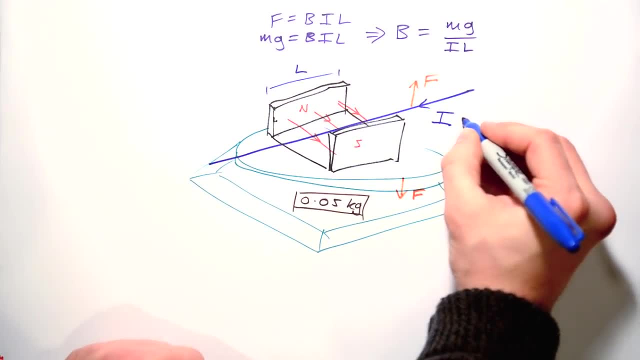 Let's pop some numbers in there Just to make sure that we know what we're doing. Let's say that we have one amp of current going through there And we know that the length of the wire That ends up being 0.1 meters. 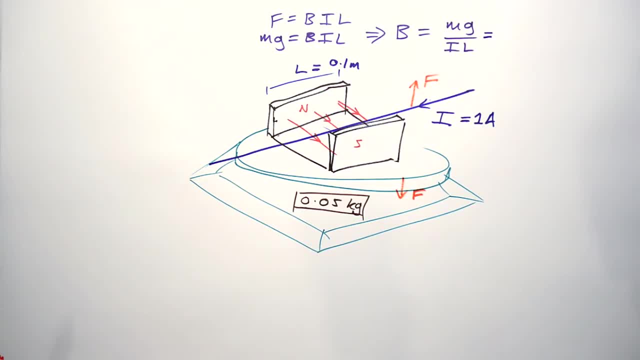 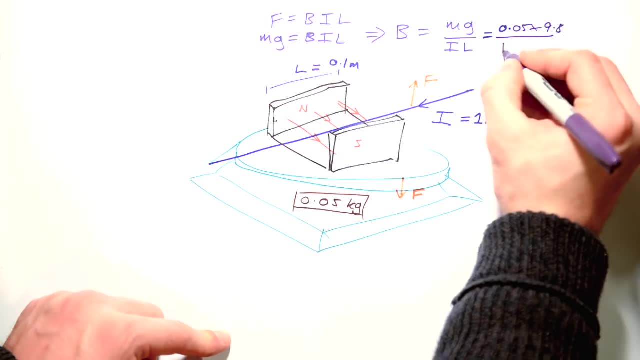 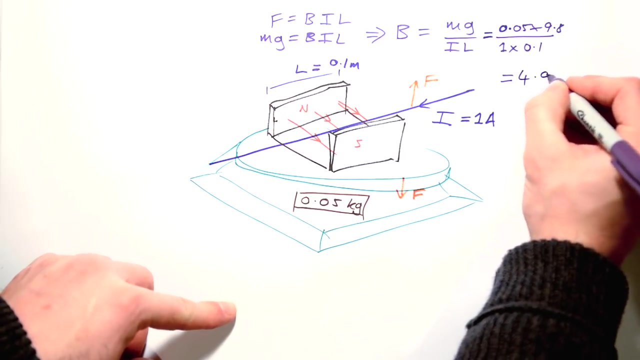 So 10 centimeters. Then we know that between these two magnets We have a magnetic flux density of 0.05 times 9.8.. Divided by 1 times 0.1.. That gives us a magnetic flux density of 4.9 teslas. 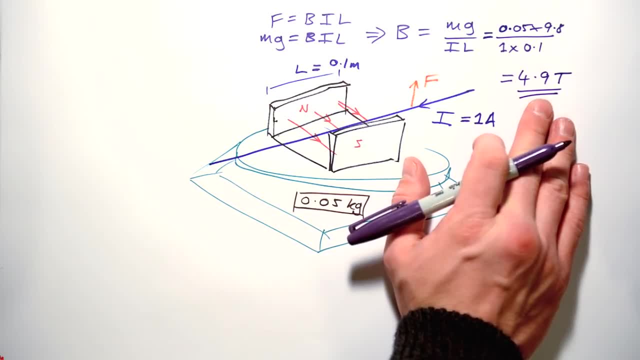 Now, in reality, this is way, way too big. Usually, when we have magnets, We have a magnetic flux density of milli teslas or micro teslas. When you do this as a required practical, As per usual, there is a way that we can find out. 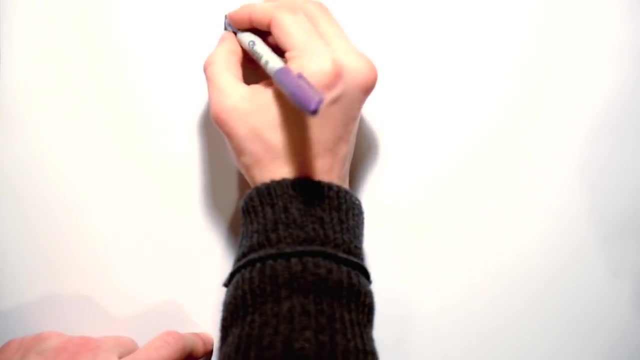 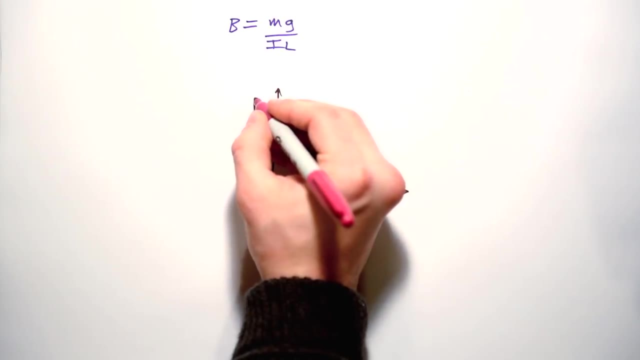 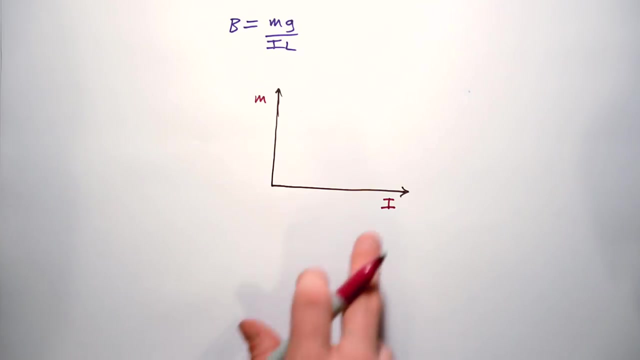 The magnetic flux density. graphically, Because our equation is: B equals M, G over IL, We can draw a graph of mass That the top band balance says that we have Against the current in the wire. You could also do length of wire.